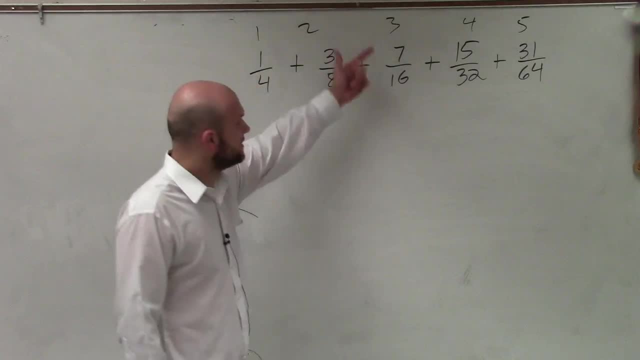 Look for addition and subtraction, right, And let's just start at 3.. And remember, we like to break this up as far as a numerator and a denominator. So to go to 3, I could add 4, right, But if I add 4 to 4, does that take me to 15?? 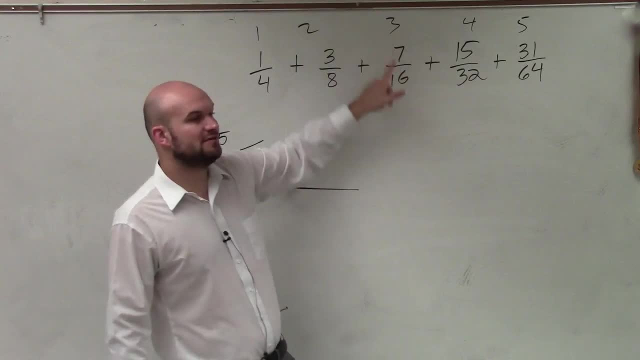 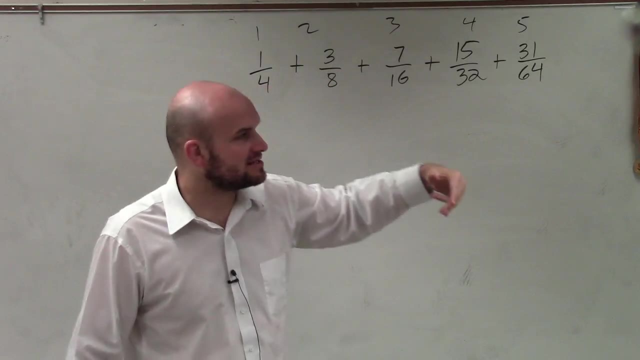 No right, Look for multiplication. Well, I can't even multiply anything to 7, so maybe let's do a combination. Why don't we multiply 3 by 2 and then subtract 2? So 3 times 2 would be 9.. 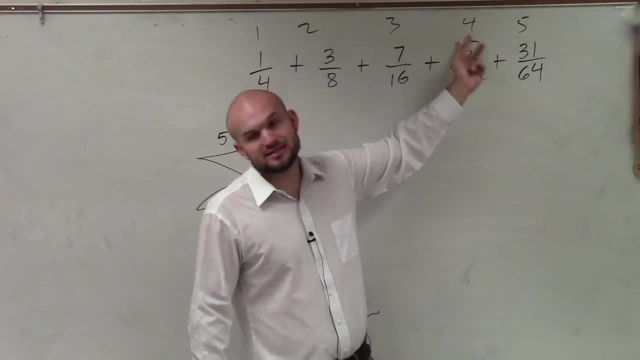 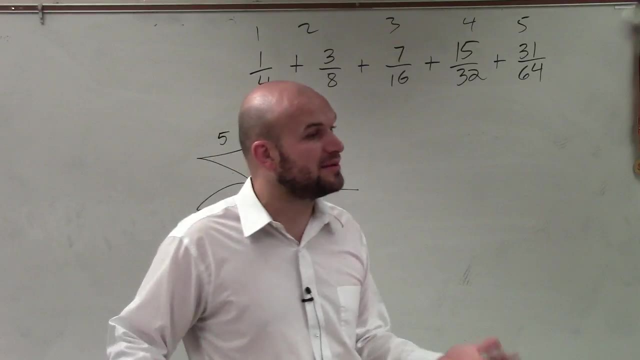 9 minus 2 is 7.. Let's do it here 3 times: 4 is 12.. Minus 2 is 10.. We need 15.. So multiplication and addition or subtraction or any combination is not really going to work. 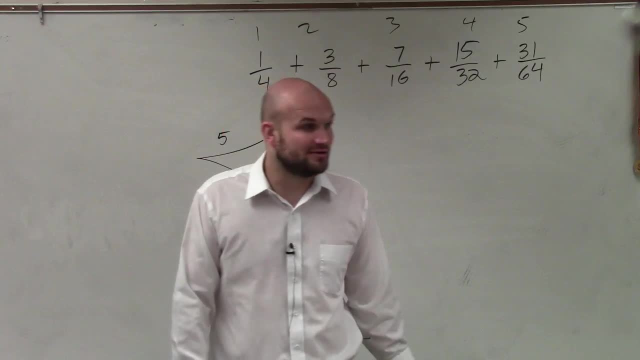 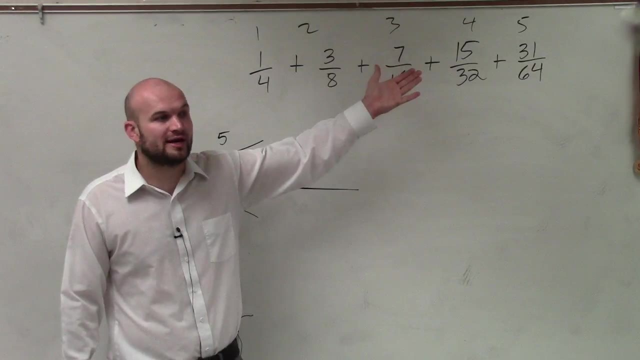 So the next thing that I like to look for is the squaring function or the power function. So let's go and look at maybe- well, we already looked at squaring it. No, we didn't, Sorry. Let's look at squaring it. 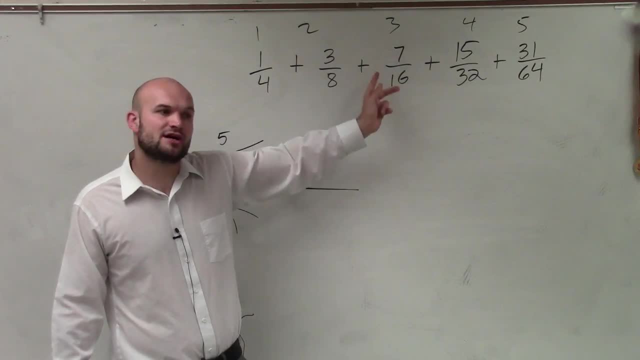 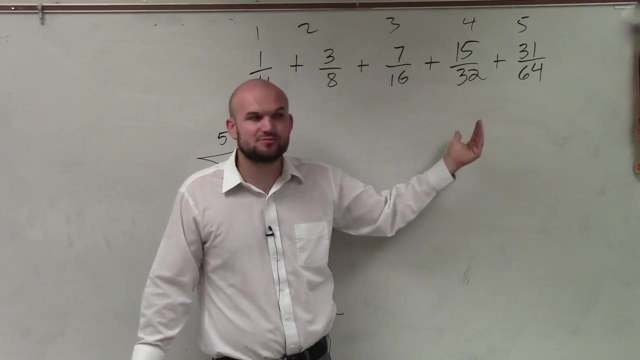 What if I squared 3,, which would be 9,, and then I subtract 2?? Well, if I square 4,, that's going to give me 16,, which is very, very close, But then I only have to subtract 1.. 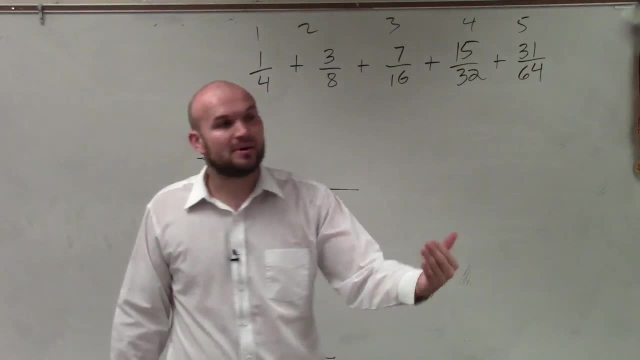 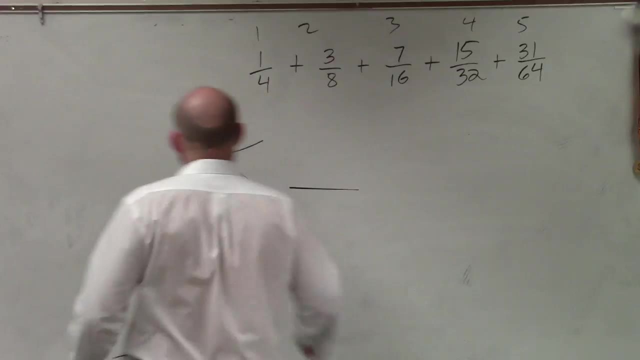 So it's not the same rule. So squaring is not going to work. But how about if I take a power? Now, what I notice about these is these are very similar to the powers of 2.. What I mean by that is, if I have 2 to the first, 2 squared, 2. 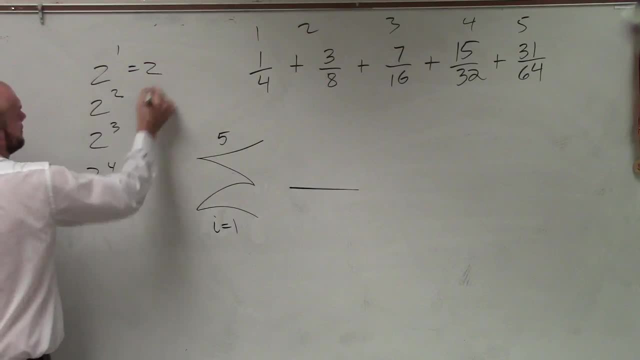 cubed 2 to the fourth, 2 to the fifth, Those are the powers of base 2.. Does everybody see that? Do you guys see how very close those numbers are to my numerators? They're the same thing, but just subtracting 1, right. 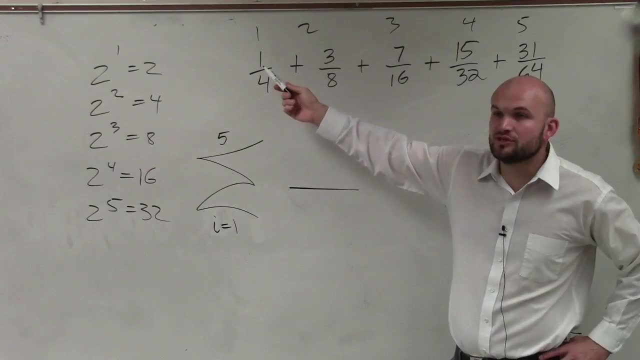 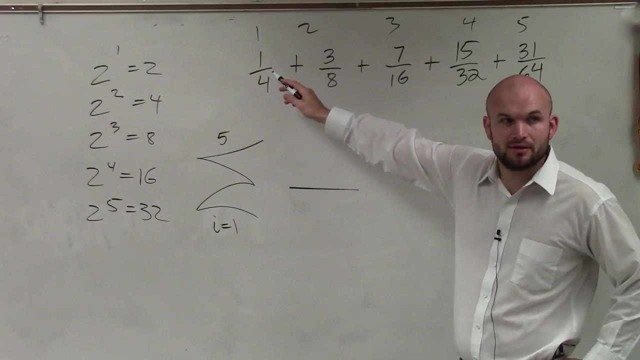 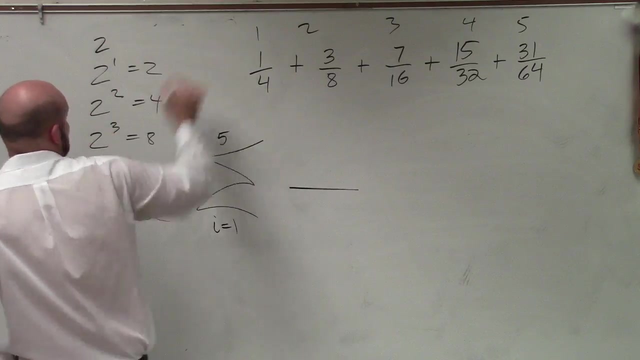 But now here, this is going to be: 2 to the first power to the first power equals 2.. So, therefore, I need to get this to be 1.. So I do know that, Oh, that can be, yeah.